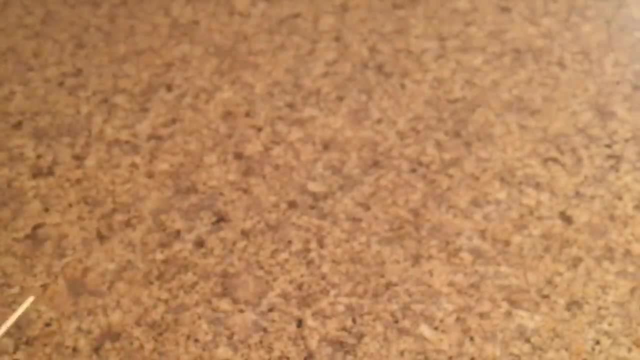 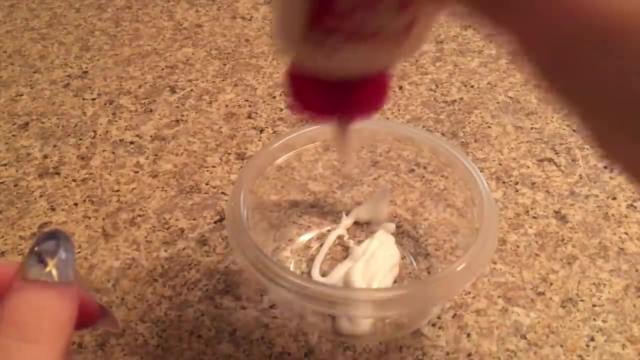 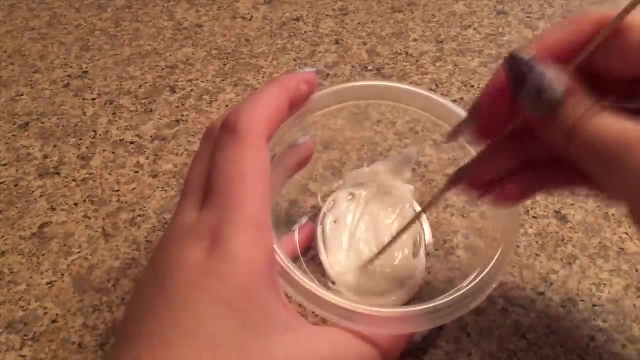 you guys will need a mixing tool. So I actually tested this recipe a while ago, but it didn't work, so I want to test it again. So I'm first going to add my lotion to my bowl, and that looks like enough, And now I'm going to take out my mixing tool and just mix it a little bit, even though 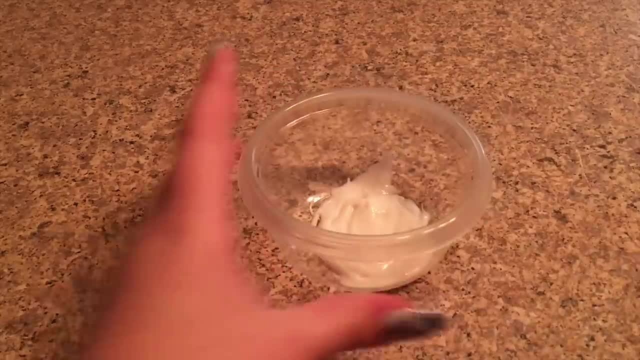 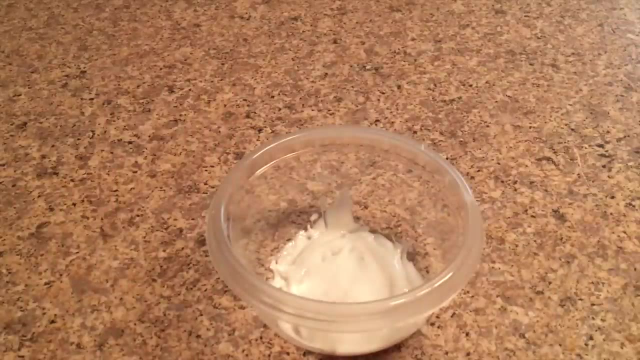 it probably won't do anything, but I want to see if it does. And now I'm going to put this into the refrigerator for about an hour and I'll see you guys in a second After about an hour. and here it is and it looks like nothing happened. but I'm just going to check, just in case. 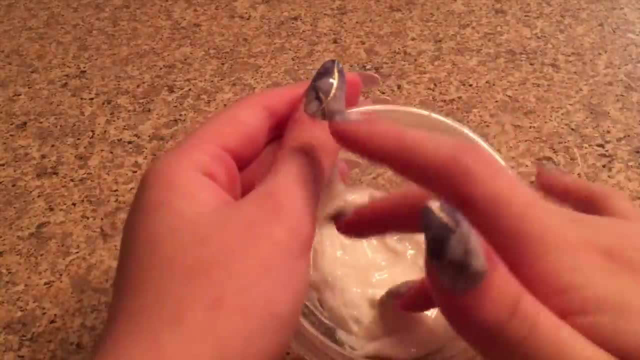 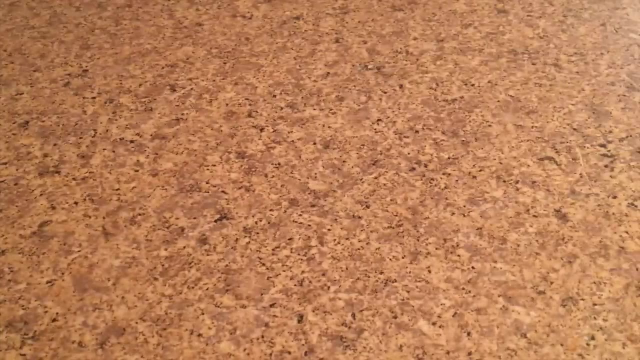 And, as I said, nothing happened. It just got really cold. But yeah, so this was unfortunately a fail, so let's move on to the next no-glue slime recipe. Okay, so the next no-glue slime recipe I'll be. 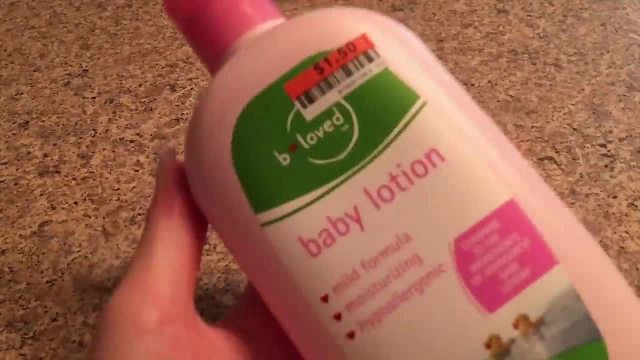 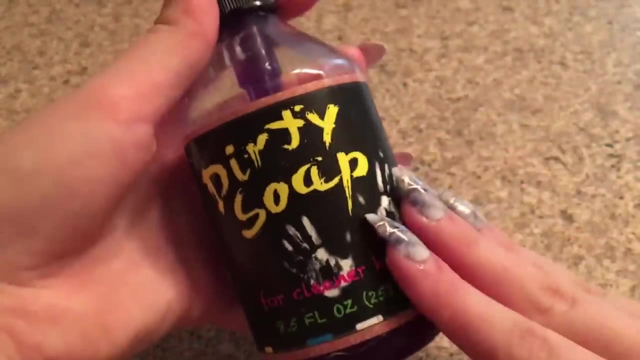 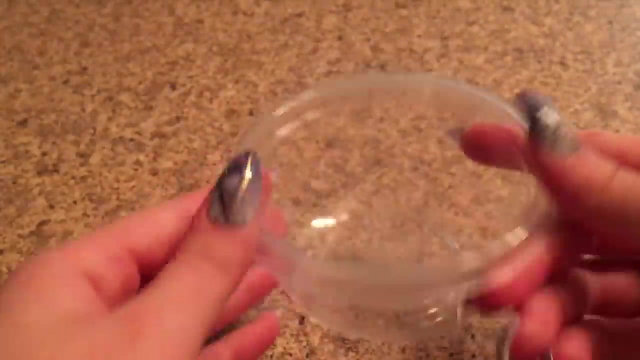 testing today is soap lotion slime. So the ingredients you guys will need to make this slime recipe today is lotion, and I'm using baby lotion. The next thing you guys will need is hand soap, and I got this one from Walgreens. You guys will also need some salt and a bowl or plate to 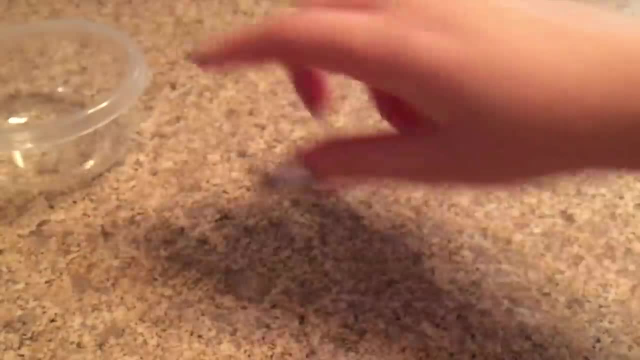 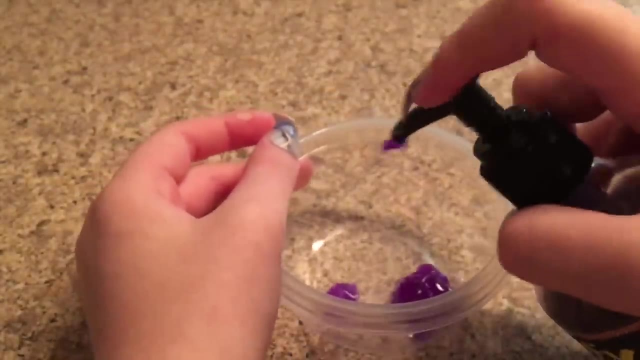 make your slime in. And, last but not least, you guys will need a mixing tool. So I actually saw this recipe on Google and it was kind of surprising to see it on there because, like, I didn't really think this would work, but I really want to test it for you guys today. 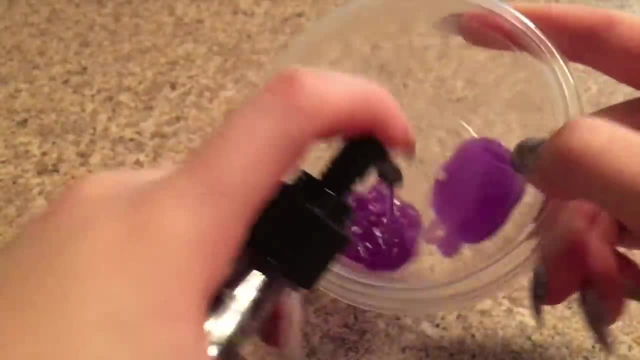 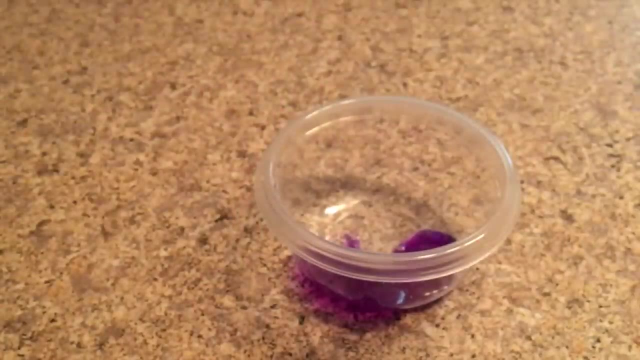 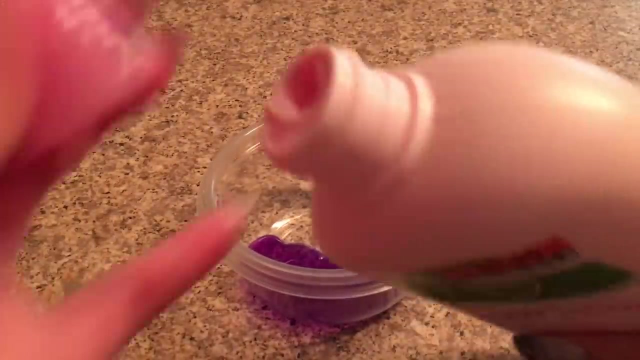 So I'm first going to add in my hand, soap into my bowl, and there it is And it smells so good, It smells like grape soda. And now I'm going to take out my lotion and it's not coming out. so I think I have to take off the lid. Yeah, I had to take off the little sticker on the lid. 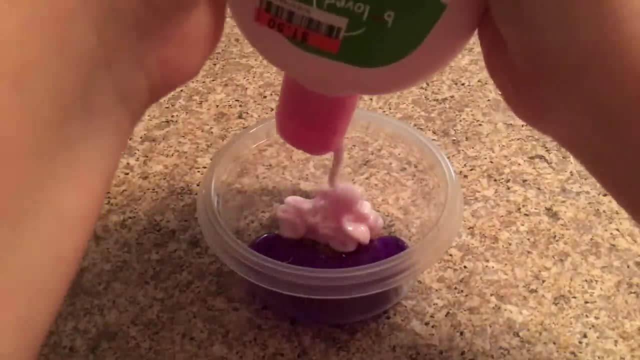 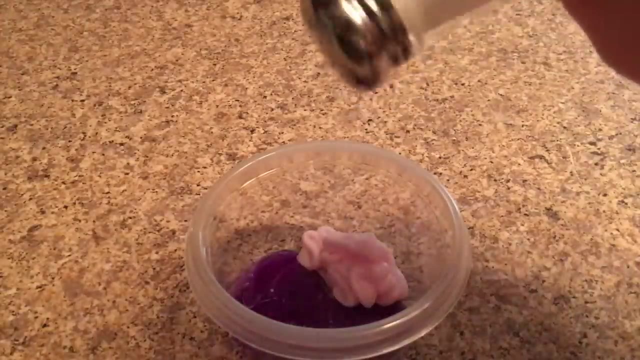 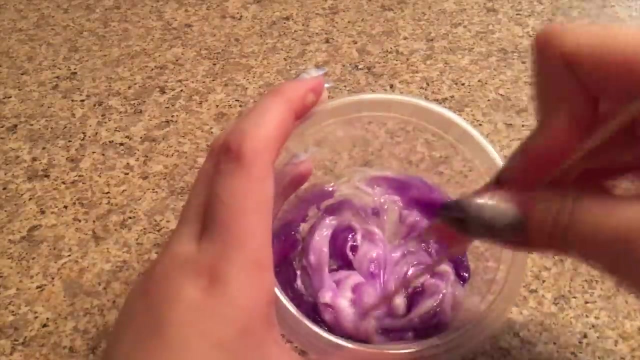 thing And I'm just going to add it into my bowl and will all the colors look really cool together. And I'm going to take out my salt and I'm going to add in a little bit to my bowl to like activate it kind of, And let's just mix this together and will all the colors look like this And I'm going 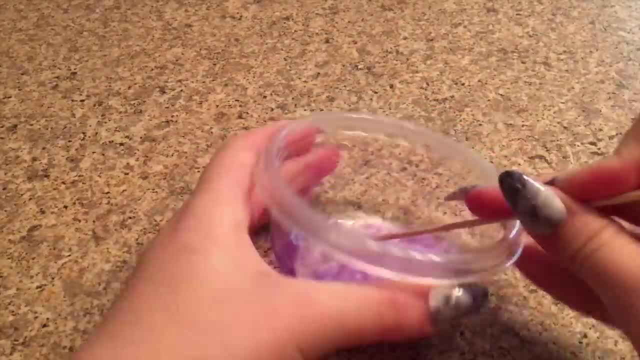 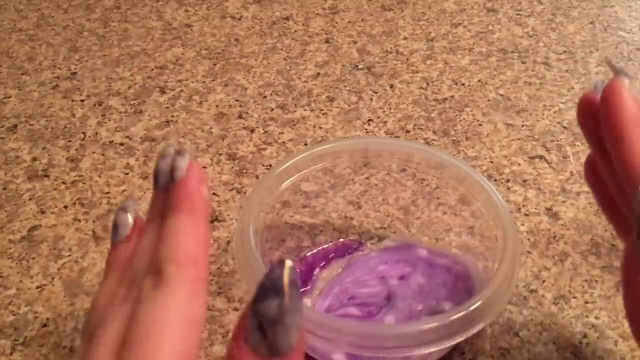 to mix this together, And I'm going to mix this together and I'm going to mix this together, And now I'm going to put this into the refrigerator for about an hour and I'll see you guys in a second. So it's been about an hour and here it is. And in between me, looking at it, I actually 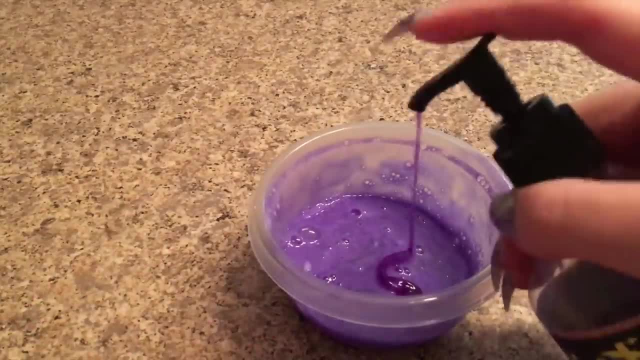 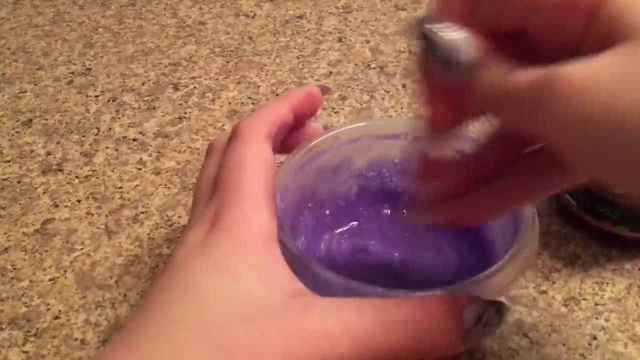 had to add more soap because it was not working at all and I was kind of upset. So I feel like soap could make it work better. And whoa, look at this. It like turned really gooey and stuff And the color changed. 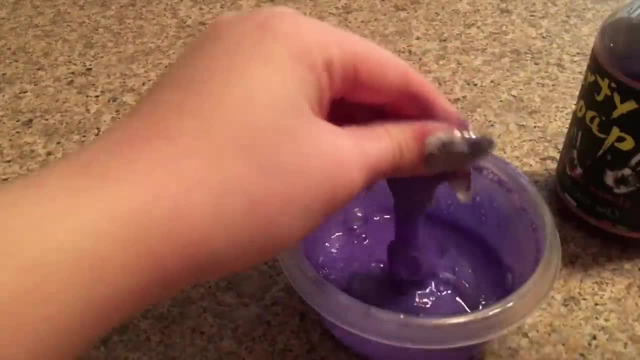 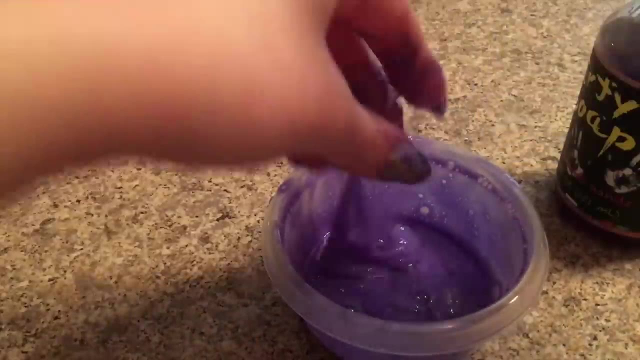 It changed a lot from the more soap I added And it's like so sticky. and it did make slime though, Like look, that's slime, But I feel like it would melt in like an hour or so. I don't know, I'm going. 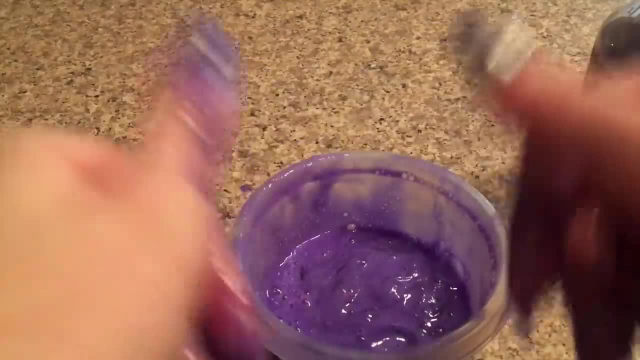 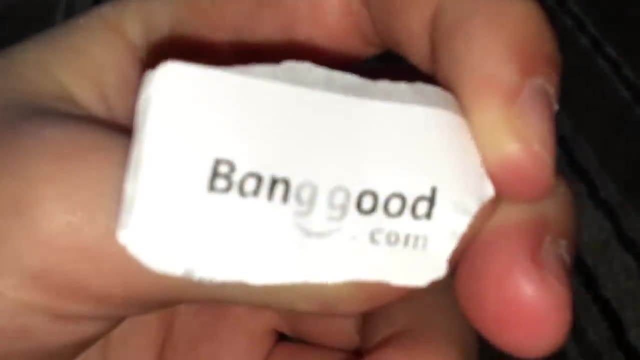 to say this was a maybe, maybe or a win-win, So yeah. so let's move on to the next no-glue slime recipe. Okay, so, before I move on to the last and final no-glue slime recipe I'll be testing today, 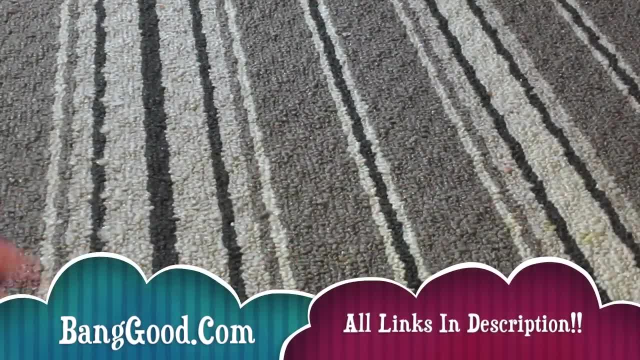 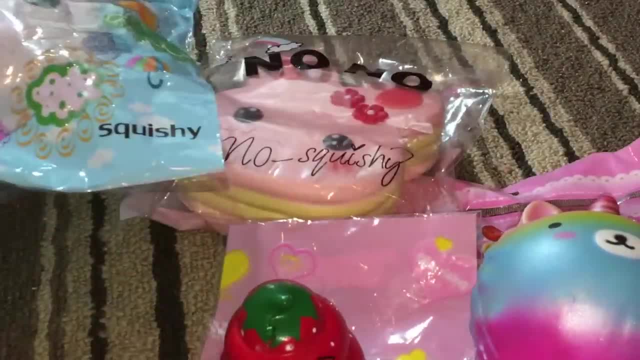 I want to talk about that, something that's sponsoring my video today. It is Banggood. Banggood is a really cool website that sells all sorts of stuff. They sell squishy-related products, slime-related products, clothing, electronics, all sorts of stuff. But today they 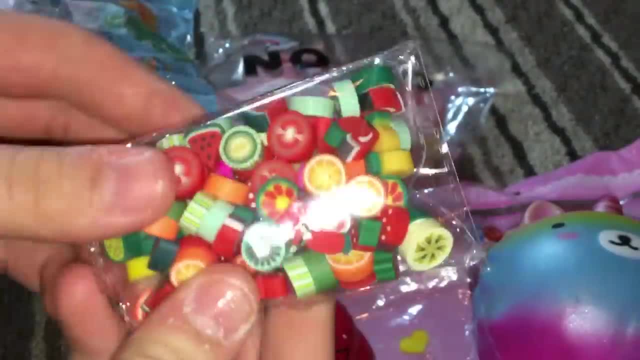 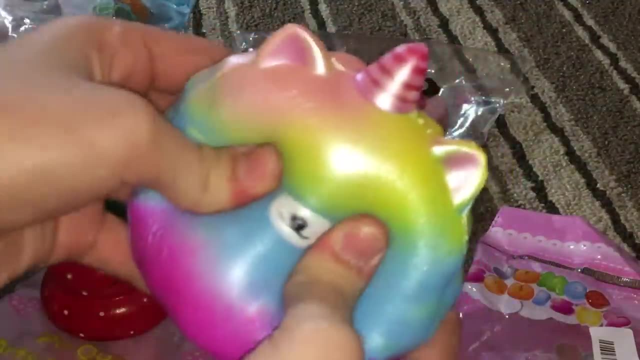 sent me a package of squishies and slime stuff. Here is a slime thing they sent me. It's like little charms to add into your slime, which is so cute. It's like fruits. Then they sent me some squishies. They sent this really cute. I think it's like a unicorn cat. It's so cute and it's. 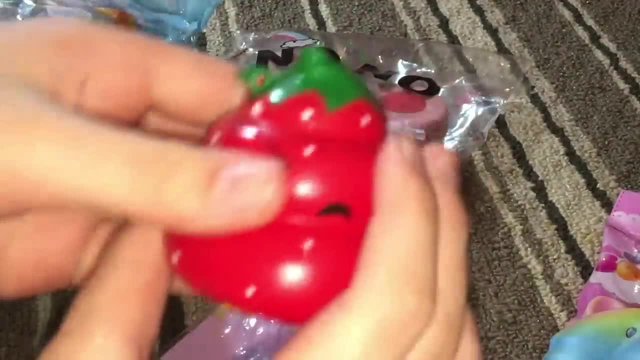 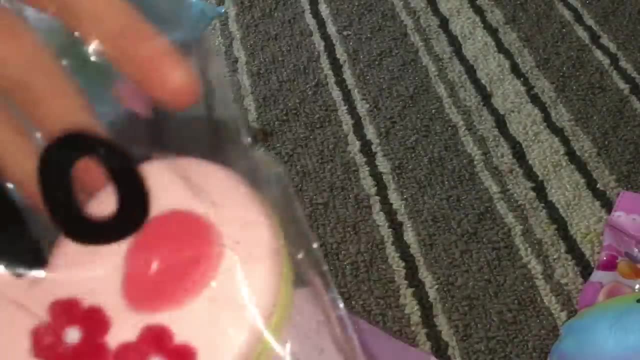 really glossy. They also sent me this like: I think this is like a tomato poop or like a- I don't really know how to explain it. They also sent me this strawberry bunny cake thing and it's so squishy and it smells just like strawberries. And all these squishies are at an affordable price. 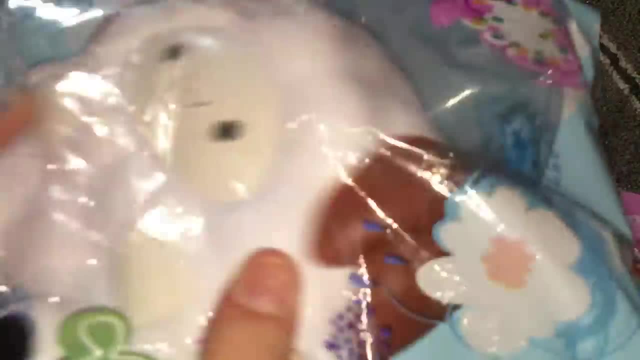 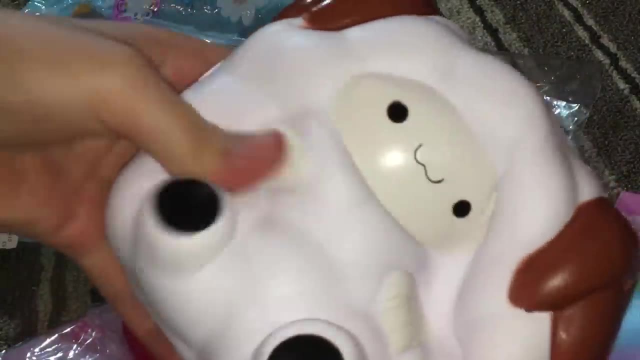 and like these are like super cheap squishies, but they- their quality- is amazing to think about, and I love the packagings too. And look at this little sheep. I have another one of these. it's like a pink one, but I'm so excited to have a white one now. And go check out Banggood. 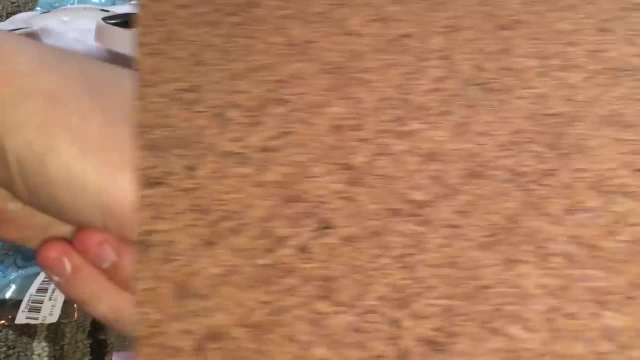 all the links will be in the description box down below. So let's move on to the next no glue slime recipe. Okay, so the last and final no glue slime recipe I'll be testing today is baby oil lotion slime. So ingredients you guys need to make this slime: 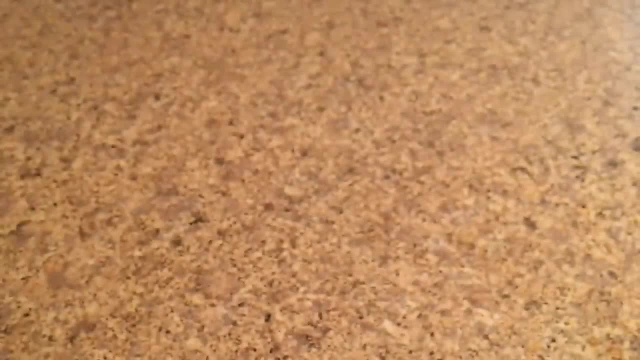 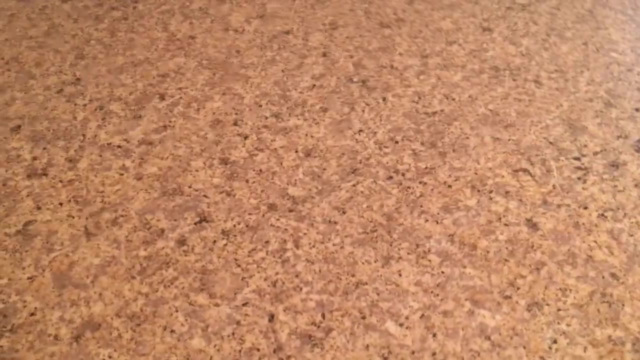 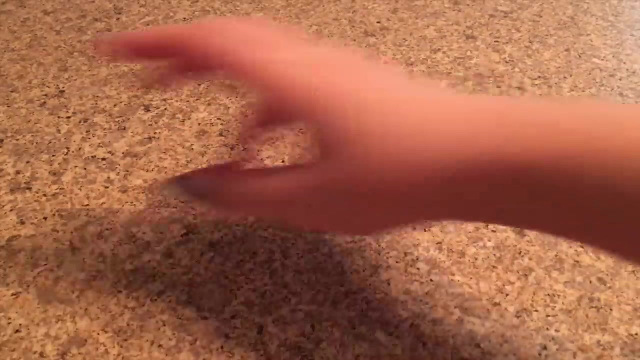 recipe today is body lotion. You guys will also need some baby oil, and I'm using this baby oil gel. The next thing you guys will need is a bowl or plate to make your slime in and, last but not least, you guys will need a mixing tool. So I never heard of this recipe, but I thought I'd try it out today. 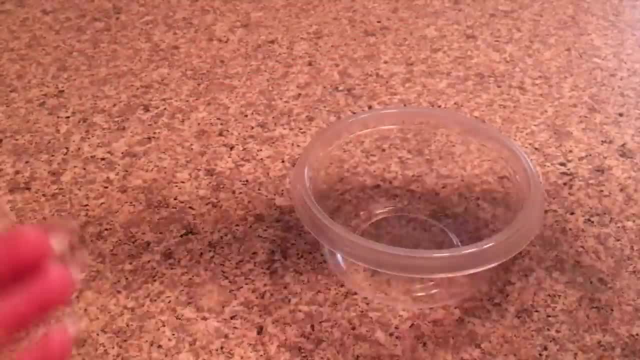 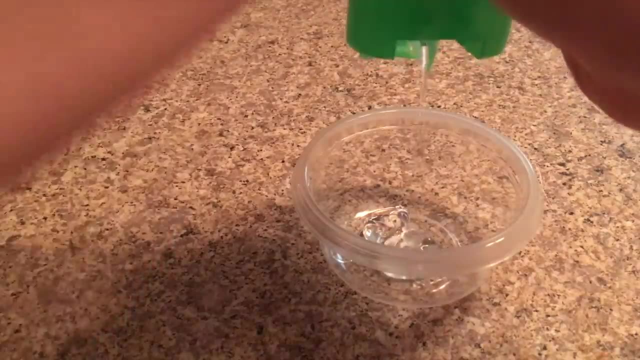 I knew of baby oil, but I actually went to the store and found this baby oil gel and I thought I could try it out for this slime recipe, So I'm going to add it into my bowl and that looks like about enough. 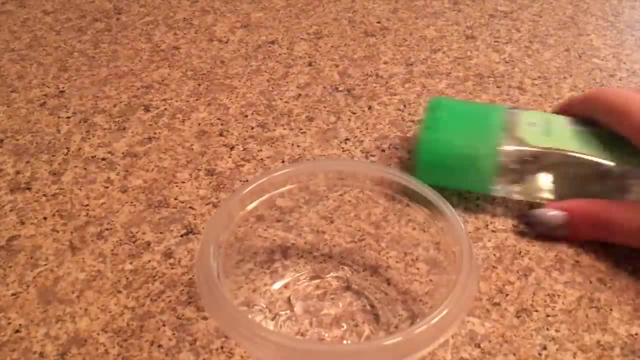 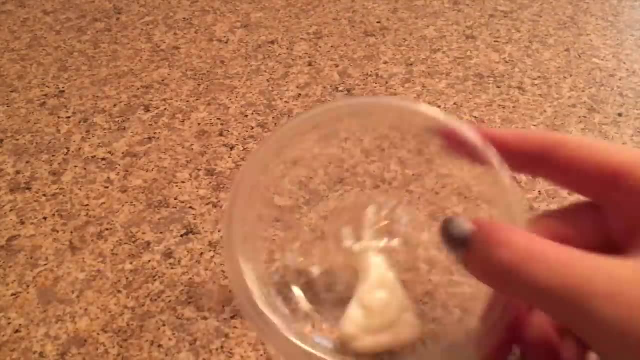 And now I'm going to take out my- oh, that just fell- my body lotion and I got this one from Bath and Body Works and it smells so good And I think this is going to turn kind of like a pink color. 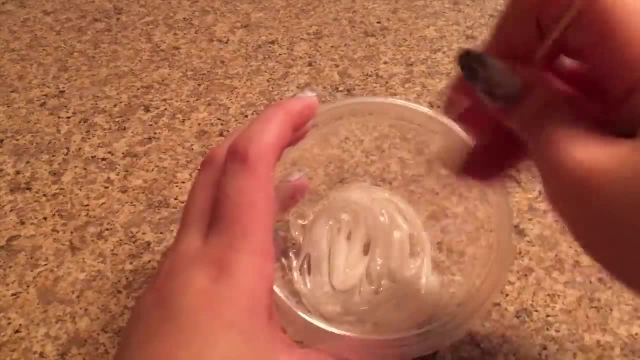 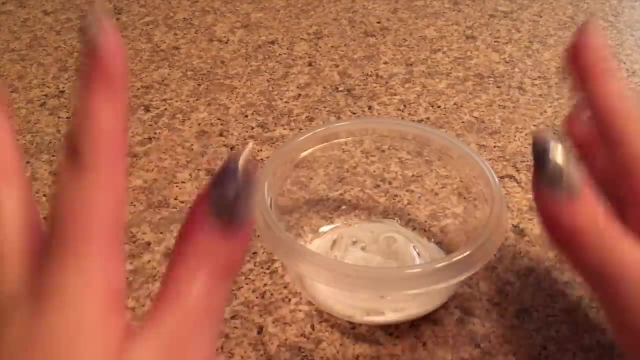 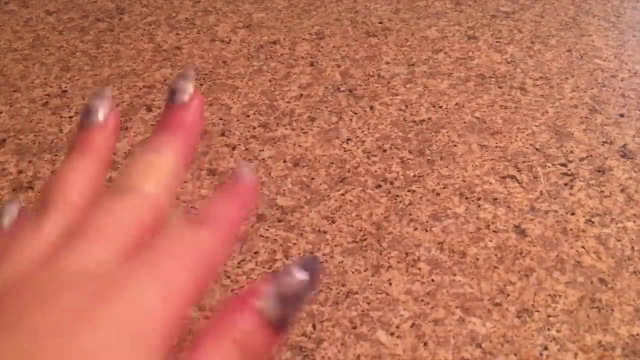 it's like a really light pink color right now. Okay, and now I'm going to put this into the refrigerator for about 45 minutes and I'll see you guys in a second. So it's been about 45 minutes and actually the baby oil caught me when I was adding some more into. 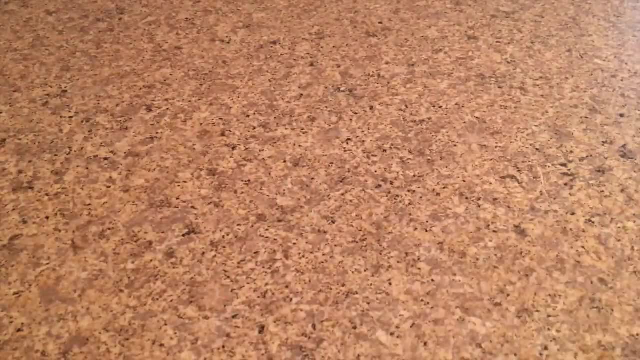 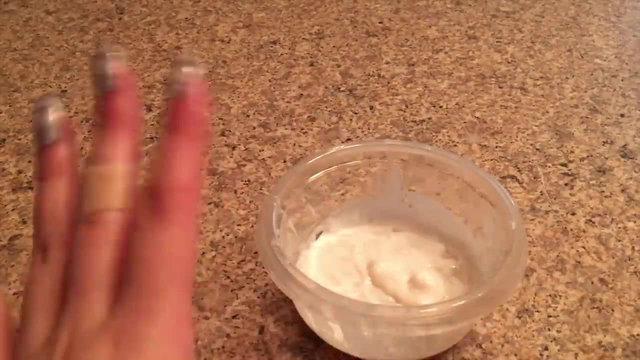 the bowl and like, just be careful when you're opening stuff, guys. But here it is, and I did add in a lot more lotion because I said before, a lot of these slime recipes don't work, so you have to add in more. 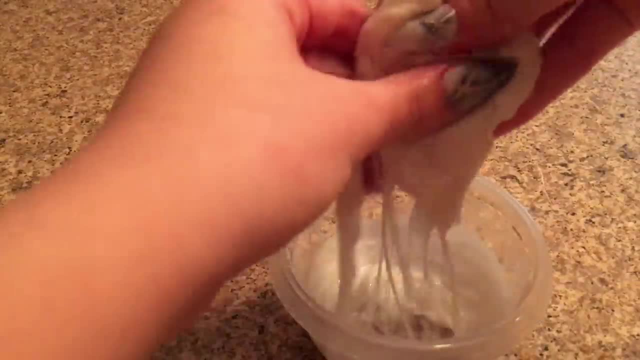 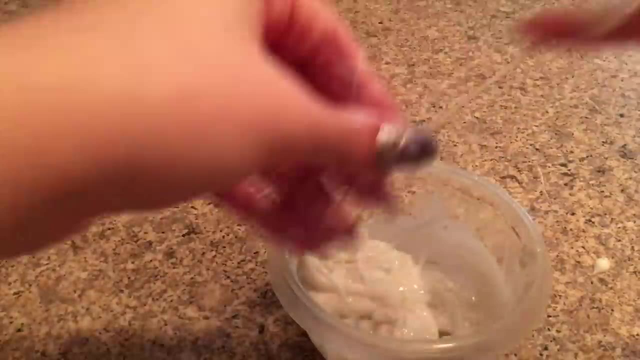 stuff And oh my gosh, look at this, guys. it like: oh my gosh, it's so sticky. It formed kind of like a slime substance, but this is really sticky right now. I feel like you could add something in to help it, so I'm gonna add in some salt. 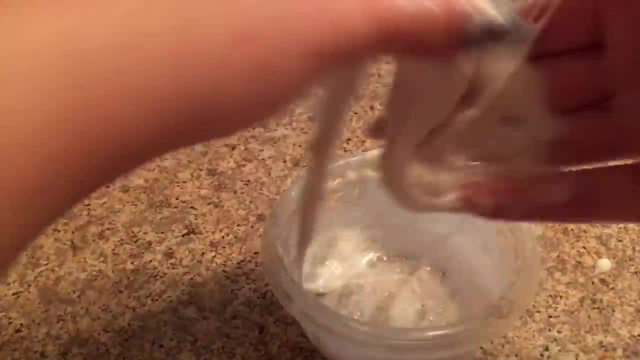 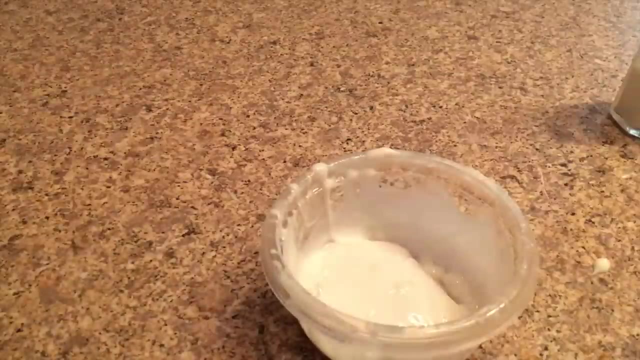 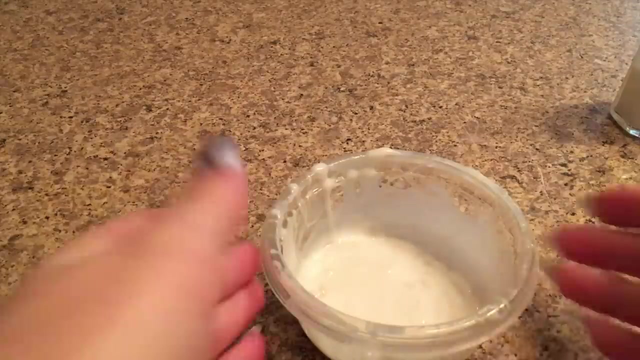 Just mix it around. It feels kind of like butter slime, but like regular slime. at the same time It's so sticky. but I'm gonna have to say this one worked today. This was a big win-win. but let me wipe off my hands really quickly. This was so sticky, So I do suggest putting into the freezer. 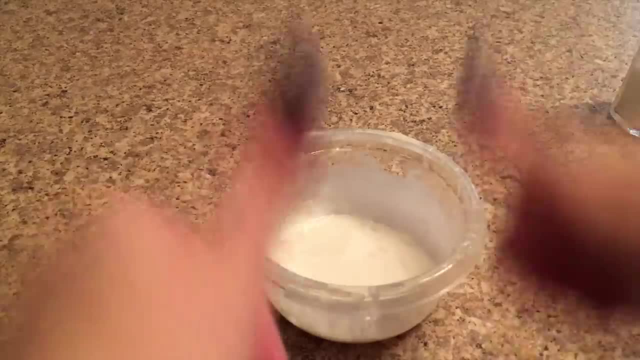 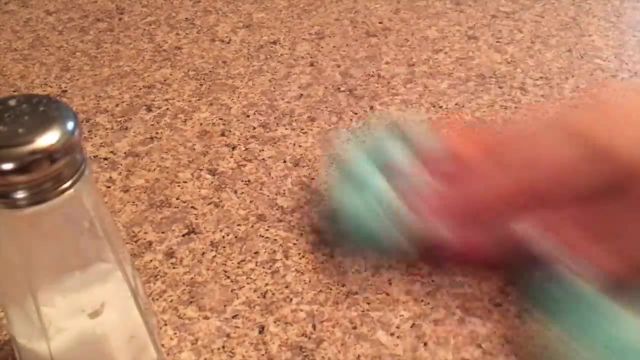 for about longer, but this did work And yeah, so thank you guys so much for watching this video today. I'll show you guys all the slime recipes that I tested and if they did good or not good. Let me wipe this off with this towel. 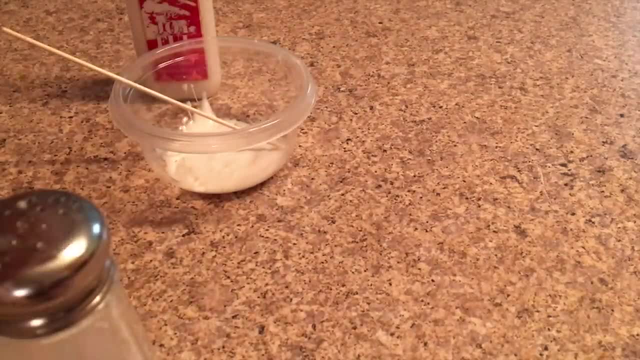 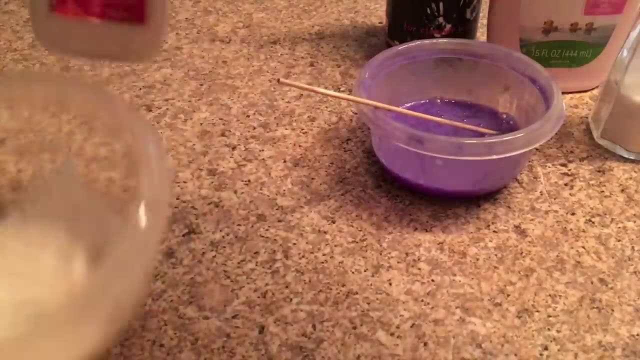 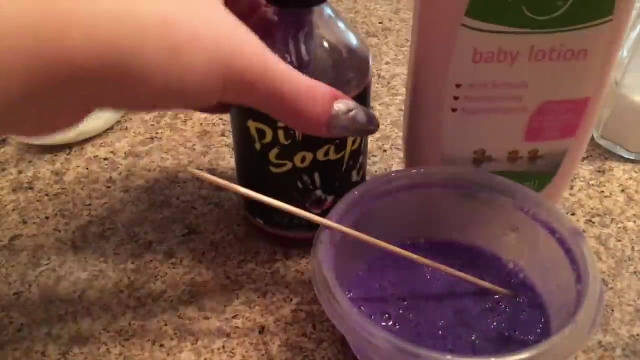 Okay, so here is the slime recipes that I tested today. So the first one I tested was the regular lotion slime, and it was unfortunately a fail, And then the second one was the hand soap slime and the lotion slime, and this was like a maybe. 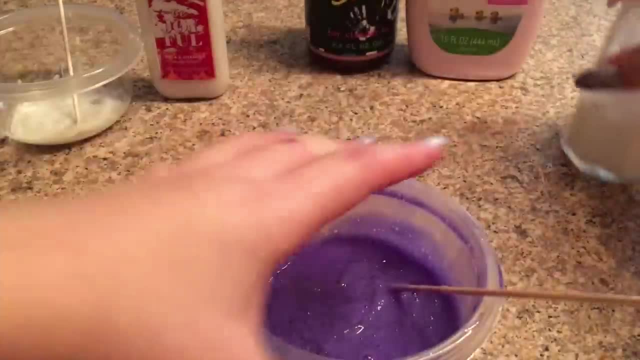 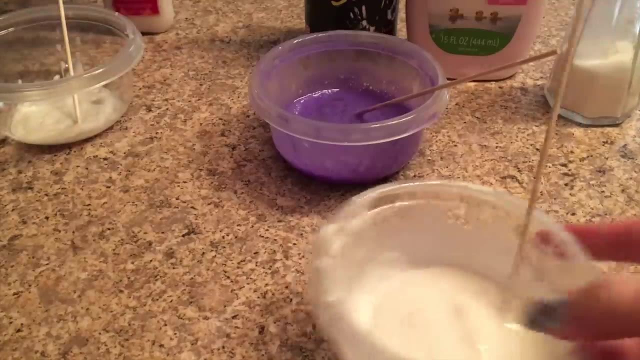 maybe because it did form something like a slime, I guess. And then, last but not least, one was the baby oil gel and the lotion slime, and this one did form like slime and I feel like if I put it in the freezer, more it would work. So thank you guys, so much for watching this video today, Please.